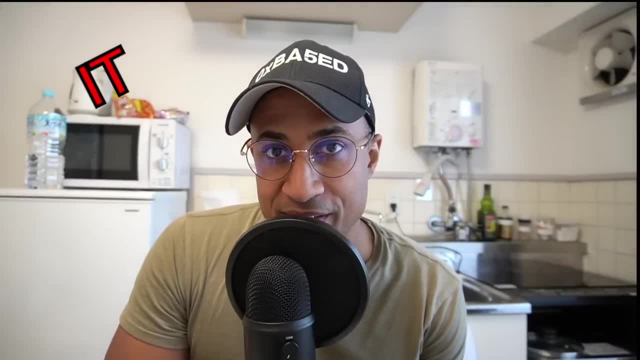 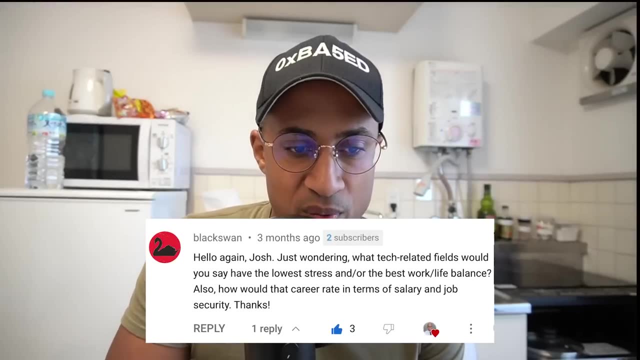 Hey everybody, Josh here, Welcome back to the channel where I talk about IT, cybersecurity, education and career things. In this video I'm going to be answering a user's question. Basically, they say: hey, Josh, just wondering what tech-related. 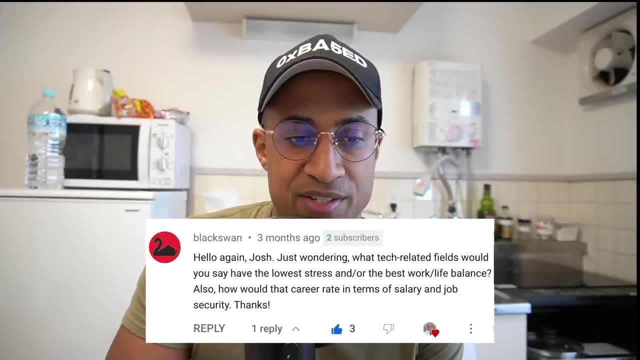 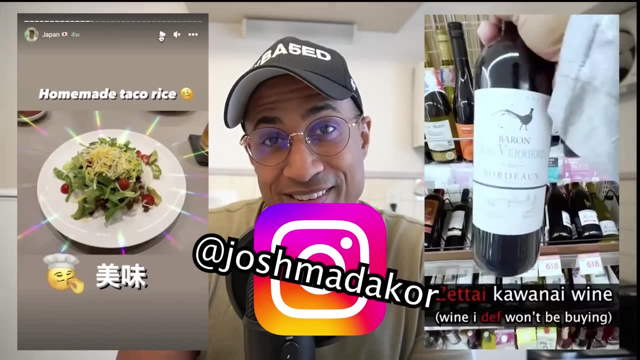 fields, would you say, have the lowest stress and or best work-life balance? Also how that career rate in terms of salary and job security. So, before we get into this, consider following me on Instagram. I post a lot there recently, a lot of high-quality content. I'm not necessarily. 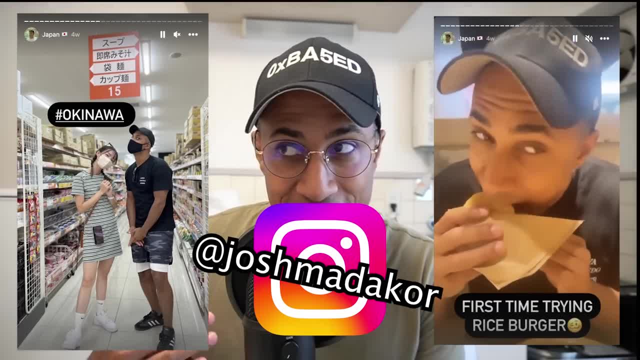 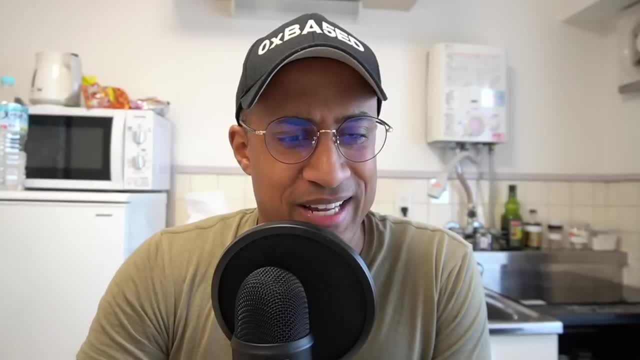 tech things, just kind of my daily life and my food. I'm eating here and like Japan scenery and that type of stuff. So check that out, Okay. so, getting right into answering this viewer's question, As far as, like, the tech-related fields, it really depends, to be honest. I'm just going to speak from my standpoint. I will say in my opinion, from what I've done, cybersecurity tends to be the worst for the lowest stress and work-life balance is okay, But for me cybersecurity tends to stress me out because a lot of the jobs I've worked have been like: 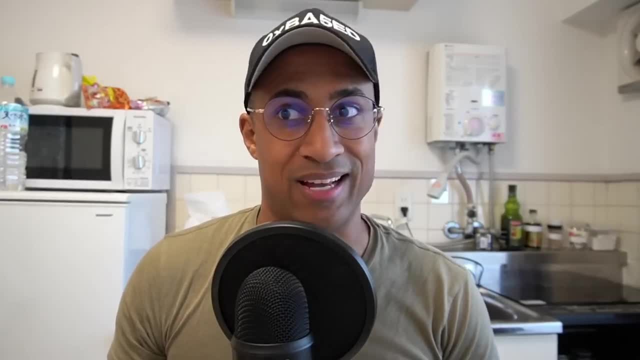 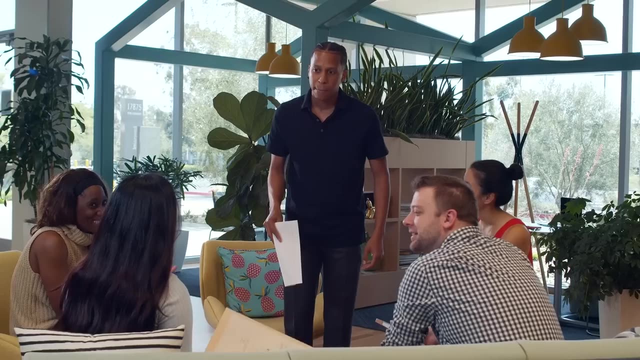 governance or risk and compliance, In order to do that job well, it relies on other humans doing their job. So I'm going to be answering that question. So, if you have any questions, where I worked, that environment wasn't good for that And people just wouldn't do their job. 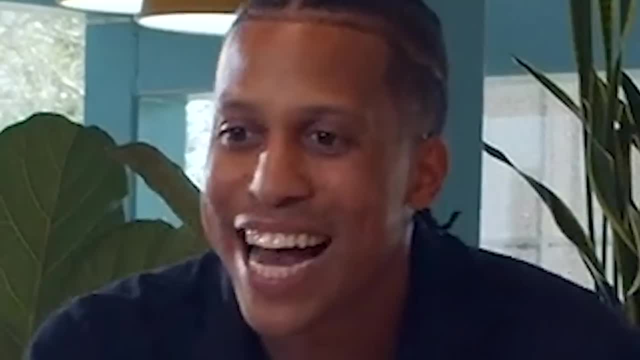 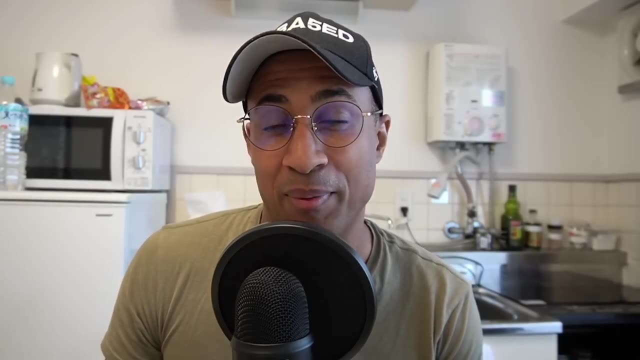 properly And as such it made my job tend to suck quite a bit. But cybersecurity is pretty good work-life balance And I'm sure if you can do something technical, depending on where you work, probably the stress is going to be lower, but it really depends. 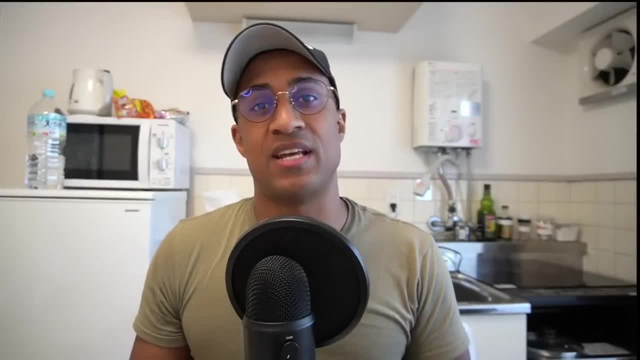 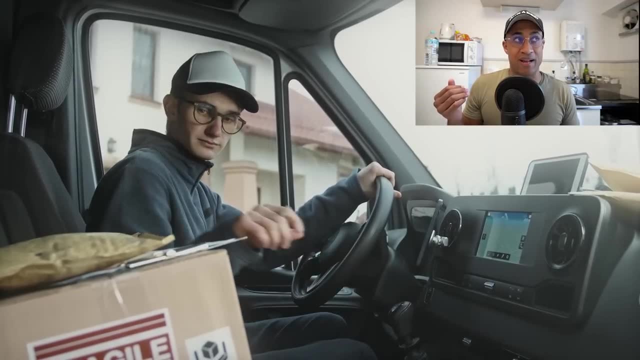 So if I were to generalize this answer, I would probably say: as far as work-life balance, you probably want to avoid the jobs where it's like you're delivering mail, So you can imagine the mailman, his job essentially never ends and he needs to spend whatever the 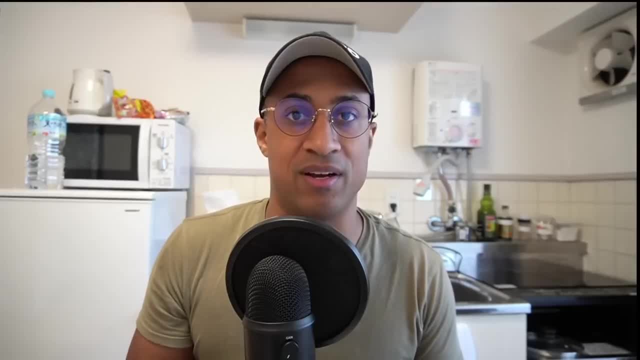 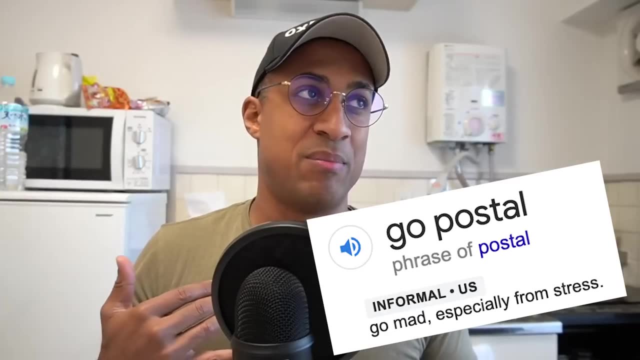 case may be eight hours every day delivering mail, or however long it takes, because the mail is always going to come. Some seasons are going to be more mail, but it's a never-ending queue. So this would be probably cloud support engineering. It pays well and it's a really 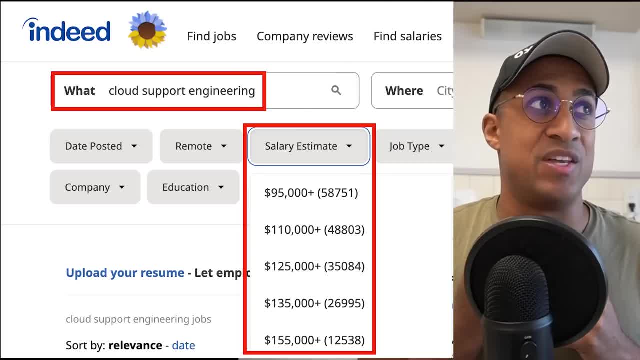 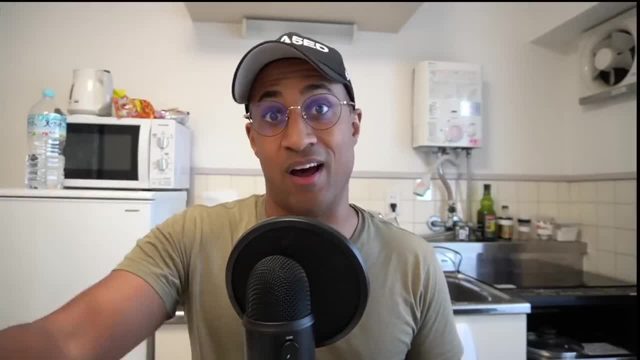 good place to work and learn stuff, but it tends to be high stress because you never really know how to solve the problems. You have to figure out how to solve every problem because they're usually difficult And you kind of have like an unending queue and it's usually like a lot of tickets to do. So you probably want to. 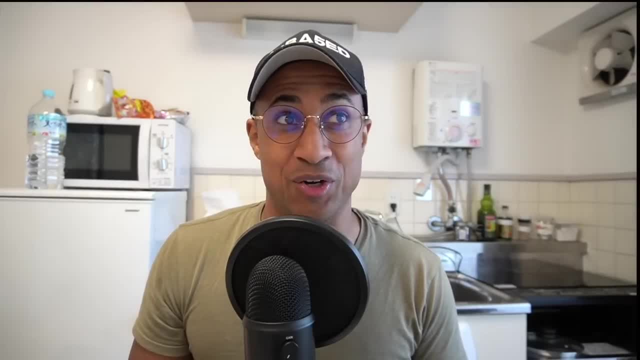 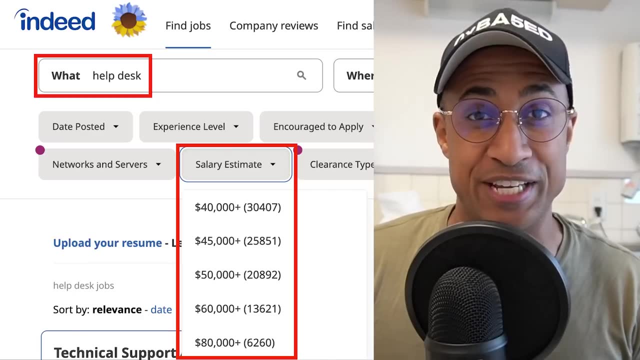 avoid cloud support engineering if you want to have like low stress and like good work-life balance. Help desk is a little bit easier. You have like a lot of unending tickets, but usually those tickets are kind of you know, much easier than cloud support engineering. So 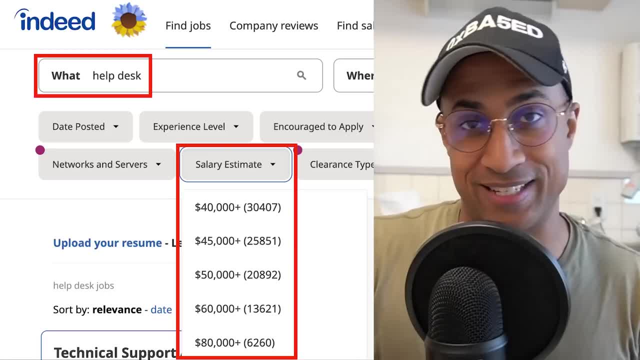 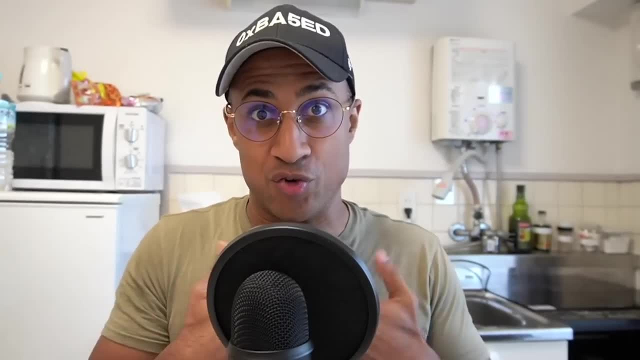 you could work some kind of support job like a help desk, like tier two escalation, or like a help desk manager or something like this- Probably going to be a little bit better- And for me, the jobs where I'm like in control of what's happening. 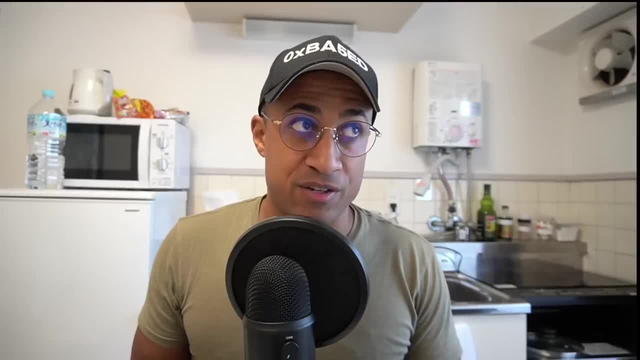 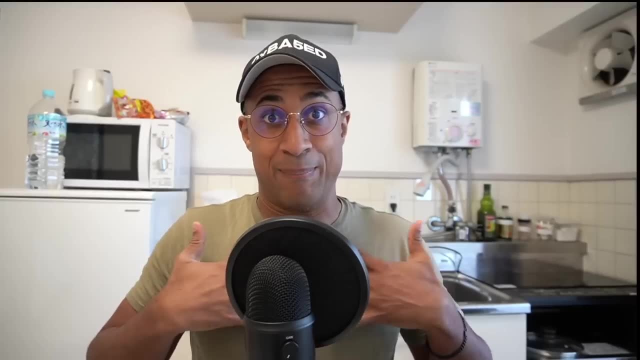 much lower stress and like better work-life balance. So my current job, for instance, I'm like a cloud automation engineer, slash software engineering. A lot of my job is most of it is like based on me, Like I don't have any roadblocks, essentially Like. 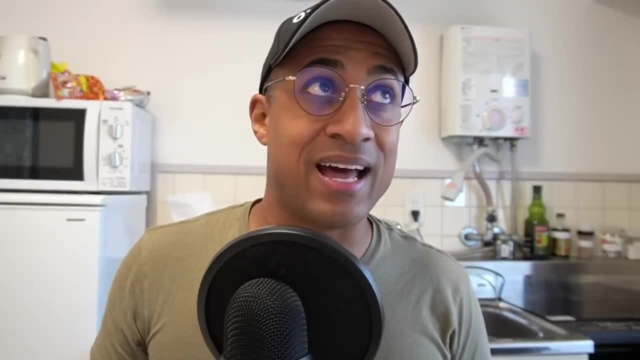 I don't have to rely on other people to do stuff And then I have like kind of an unending queue, like a never-ending list of stuff to do. but I'm really good at regulating it, So I kind of just 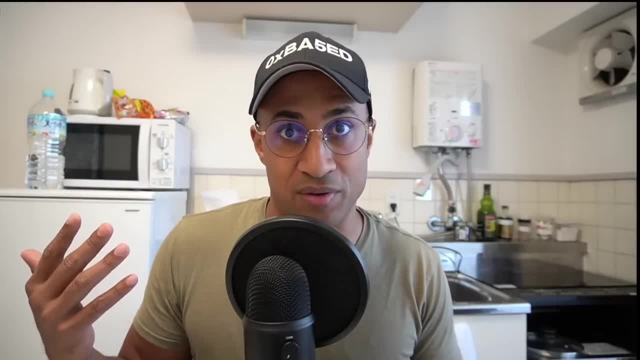 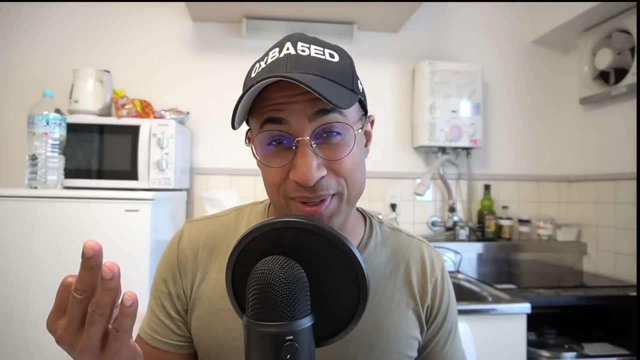 do a certain amount every day and stop, and no one bothers me. So that's like really nice. So, generally speaking probably say like the best work-life balance, the lowest stress and the highest salary, is probably something to do with coding, like software engineering or web development, or 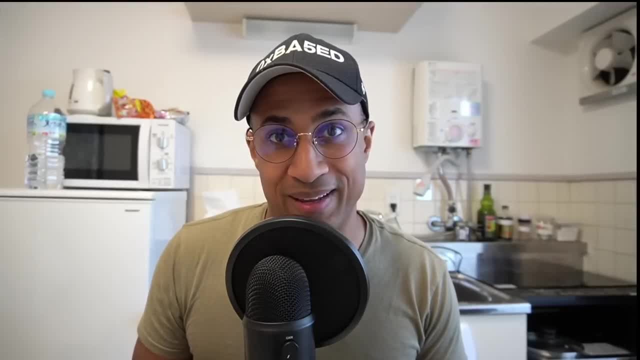 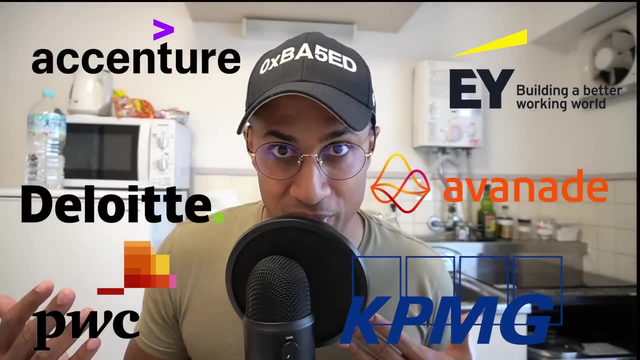 something, Of course, you don't want to, you don't? you probably don't want to work for a consulting firm like Accenture or someplace like this, because they're just going to abuse you and make you like work. you know maximum amount because, for whatever reason, so many people want. 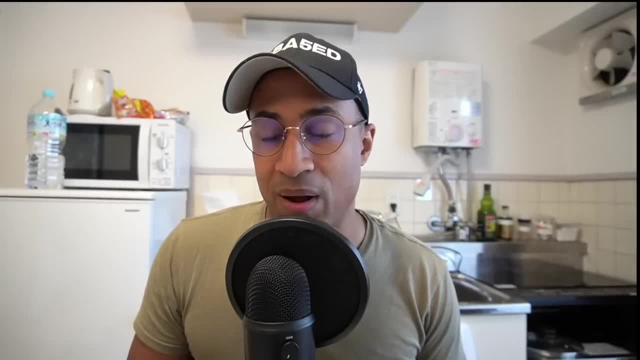 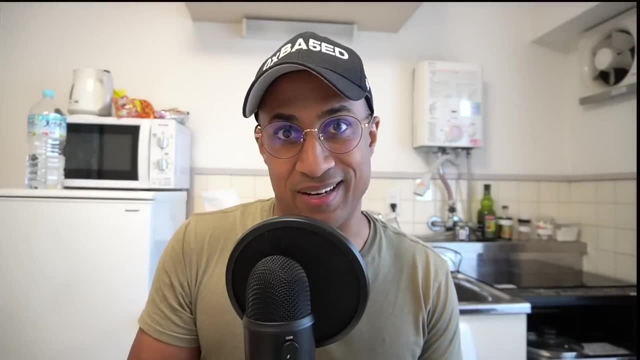 to work there, So they just like work you to death. Don't be a consultant, But probably, probably some kind of knowledge-based work that's highly skilled is going to give you the highest salary, best work-life balance and lowest stress. 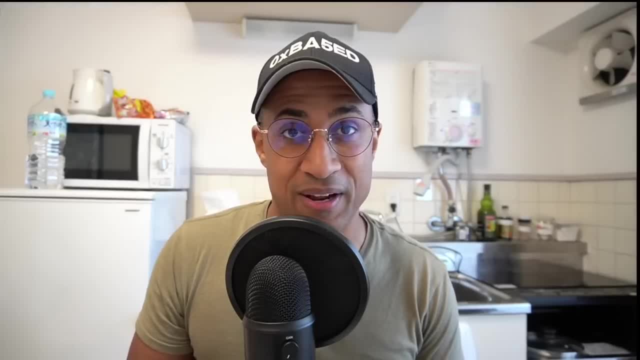 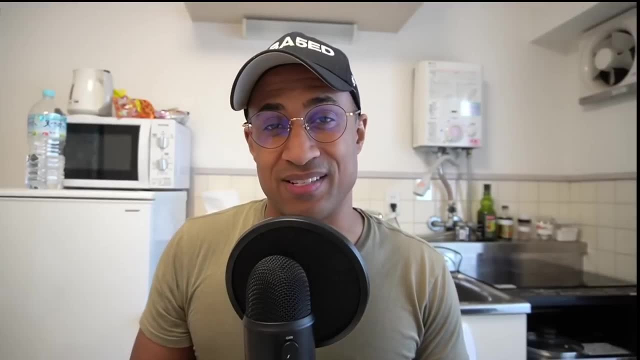 So probably software engineering or coding or something like this. right, I'd probably say, like cybersecurity and normal, you know, IT operations and system engineering is probably tied. It really depends. Like I know I'm going to say, cybersecurity probably loses out because a 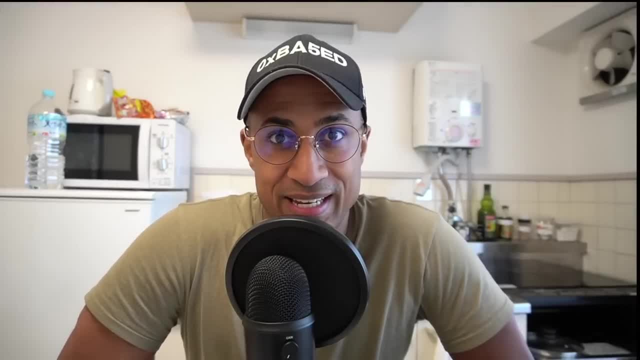 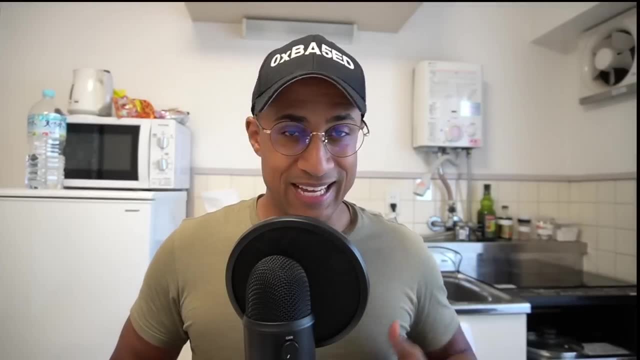 lot of the stuff in cybersecurity is incident-based and has some kind of time constraint on it, Like you need to respond to incidents in like a certain time period a lot of the time and it's like kind of out of your control, Like if something happens or a breach surprise. 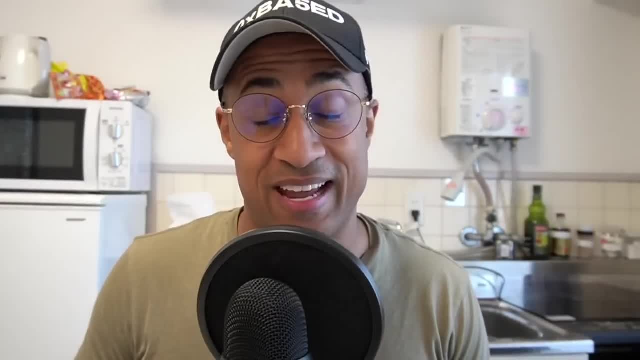 you have a bunch of work and you just can't do it. So you know that's, that's, that's, that's, that's not going to do anything about it, You just have to. you just have to handle it. Also, cybersecurity: 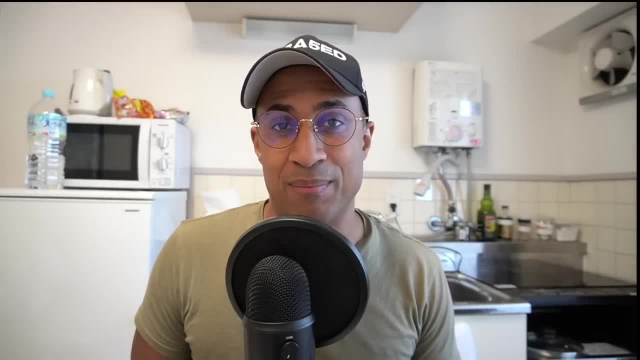 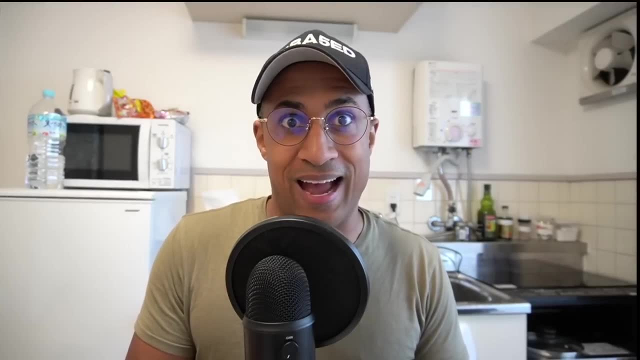 especially like, especially defensive security requires, like, a lot of collaboration, a lot of like behavior modification of other employees. You have to, like you know, get them to practice good hygiene and you're constantly like technologically babysitting people And 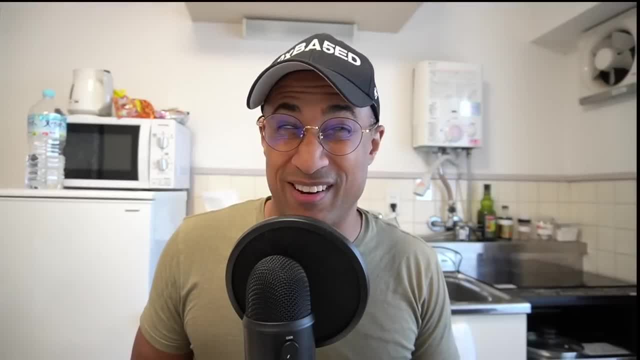 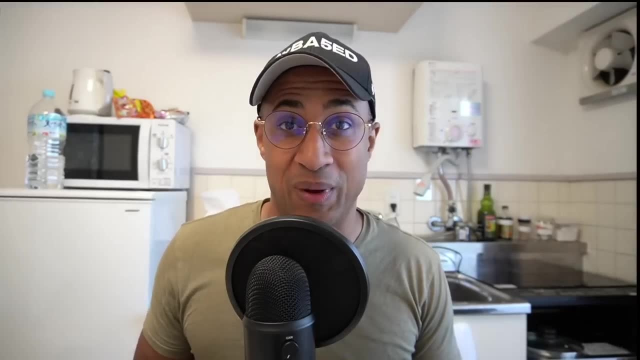 you know. if they're you, it's like hurting cast a little bit. So cybersecurity is probably not that. I don't know You. let me know what you think in the comments section. I don't really think cyber is like that great. to be honest. It pays really well and it has. there's a reason. 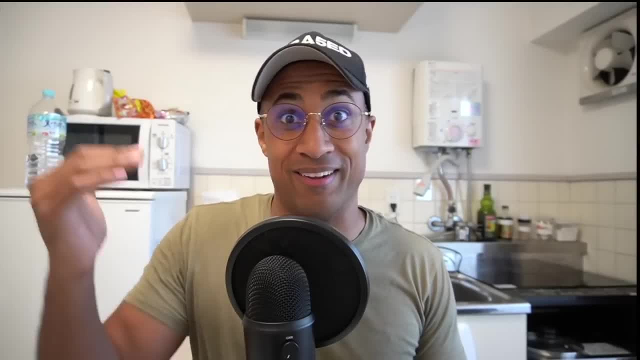 for that. A lot of people who can do cyber like either require a lot of money or they just don't do it like, like me, for instance. And I would say, like you know, general IT like sysadmin. system engineering type thing. that's probably middle of the line, because a lot of your work is knowledge-based. When you get to that level, say, you're like a cloud admin. you're just managing resources for a company. It's not like you have an unlimited list of like tickets coming. 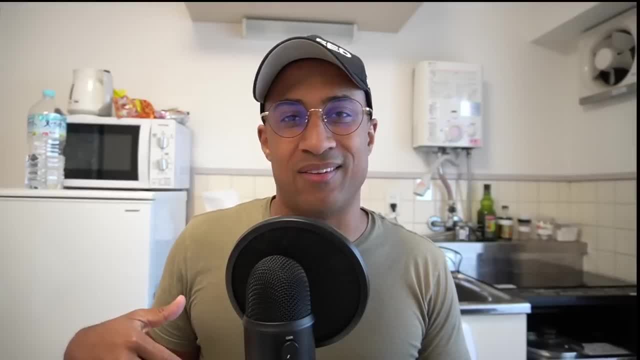 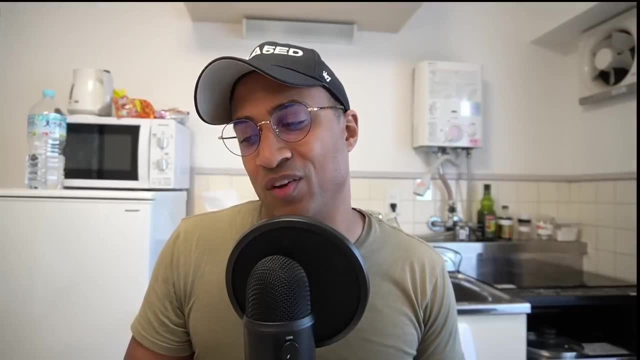 your way that you have to deal with. You probably have like projects that you do and a lot of which are kind of reliant on your own sufficiency And like how well you organize, like execute the project. So probably you know sysadmin. probably middle of the line. Cyber security- probably worst, to be honest, Probably worst. most stress because so much stuff is out of your control. And then automation: that is probably like the best of all worlds. I guess I would advocate for coding if you're into that. 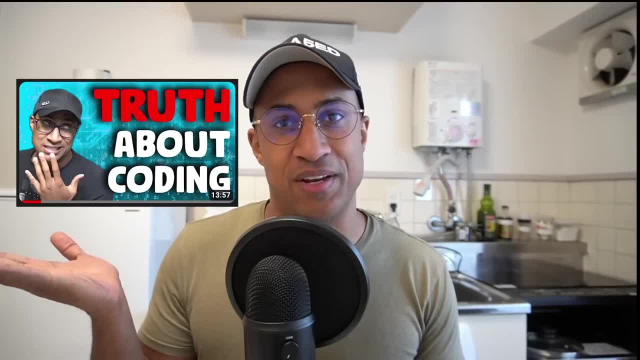 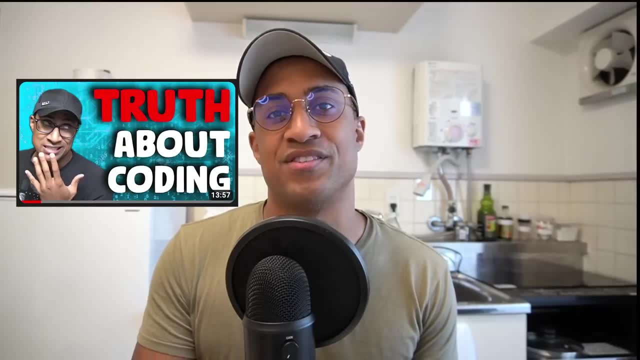 If you're one of those people who are, like, really scared of coding, watch this video: The Truth About Coding. I kind of talk about it and demystify it a little bit. It's not as hard as you think it is and you don't have to memorize anything. It's just a matter of understanding and 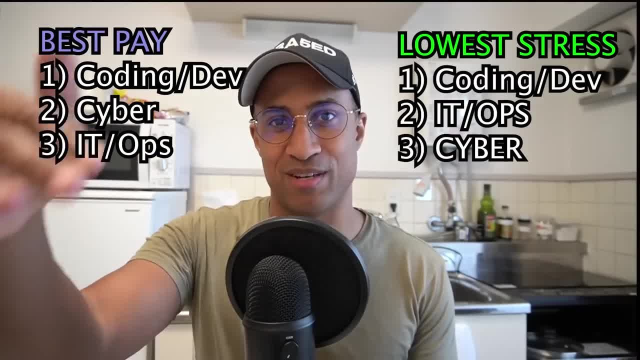 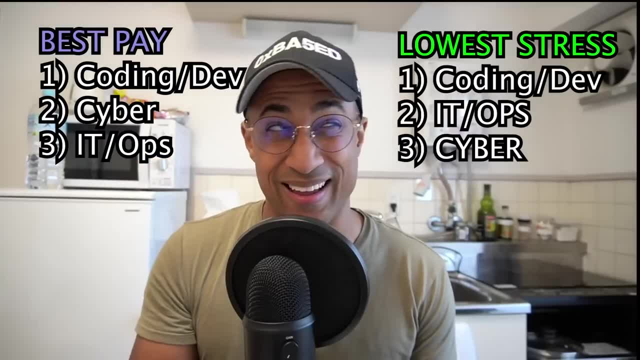 practicing, So coding. number one, normal IT, sys operations. number two: probably cyber security. number three, Although cyber pays more than system, like you know. normal IT, I guess, But I, you know I don't really like that much. Yeah, that's all. Follow me on Instagram. I try to post. 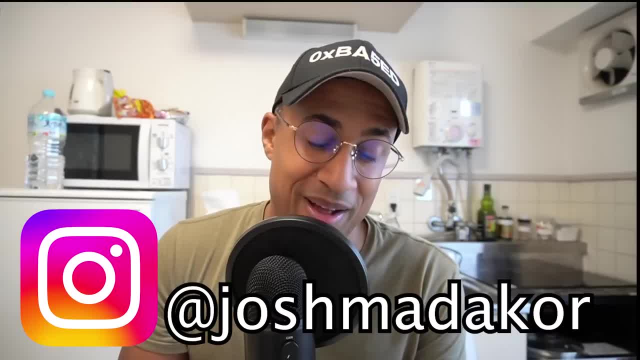 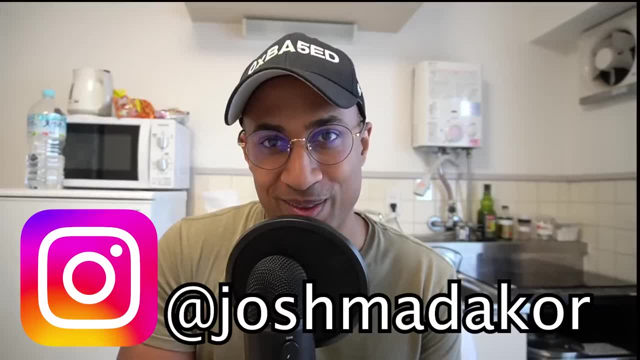 a lot there, as usual, a lot of food and Japanese things. I'll try to post much more interesting content. It's pretty good now, but we're working on trying to make Instagram better, So you know, follow me on there. I really appreciate it. 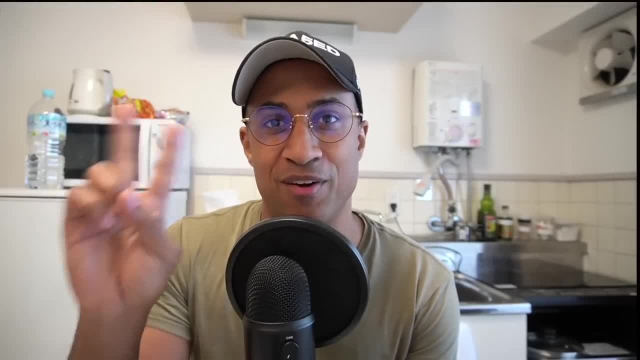 Thanks for watching, as always, and we will see you in the next video. 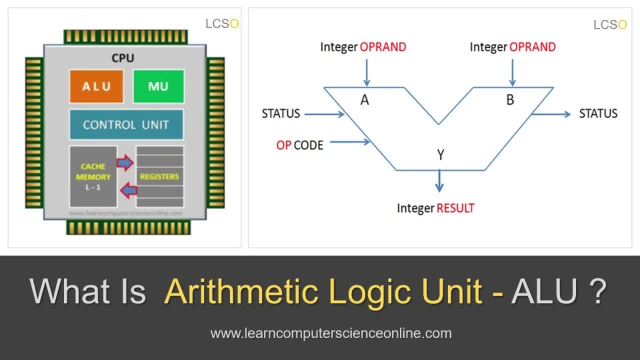 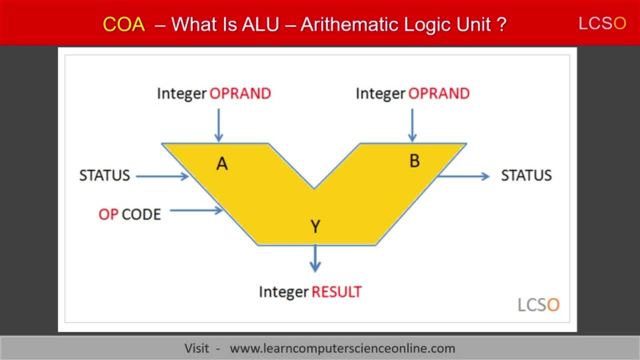 Welcome to learncomputerscienceonlinecom, and in this video we are going to discuss what is an arithmetic logic unit. Let us first start with a brief introduction. The arithmetic logic unit is commonly abbreviated as ALU in the computer jargon. 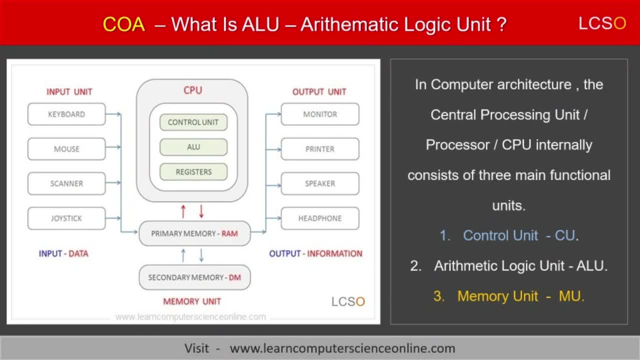 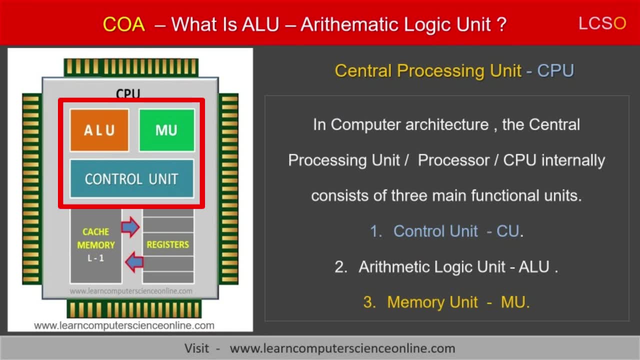 The ALU is an internal component of the microprocessor architecture. The microprocessor components can be basically grouped into three functional units. These three functional units of the CPU are, first, the control unit, second, the arithmetic logic unit and third, the memory unit.